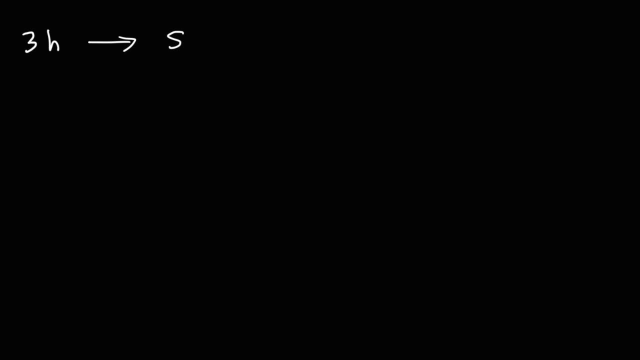 This is a two-step conversion process. You need to know that one hour is equal to 60 minutes and one minute is equal to 60 seconds. So those are the two conversion factors that we need. So we're going to start with three hours And first we're going to convert hours into minutes. 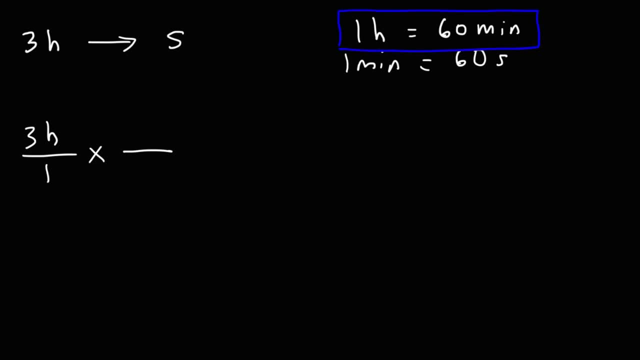 So, focusing on this conversion process, we're going to start with three hours Conversion factor. Which part of that equation should we put on the bottom? The one hour part or the 60 minute part? What would you say? Now? we want the unit hours to cancel, So we're going to put this portion, I mean. 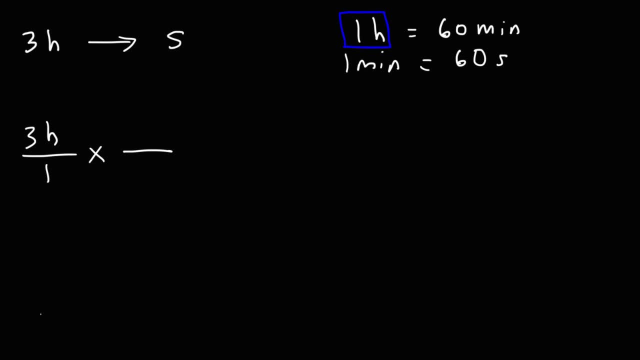 excuse me, that portion under the denominator, And then the second part will have the other side of the equation, That is, the 60 minutes. You want to set it up in such a way that you can convert hours into seconds, So we're going to start with three hours. 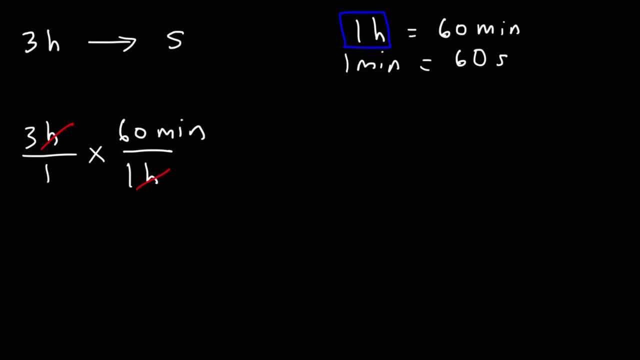 That the unit's hours cancel. Now our next step is to convert from minutes to seconds, So we're going to use this conversion factor to do so. So what should we put on the bottom? Notice that we have the unit minutes on the top here, So we want to put this on the bottom. 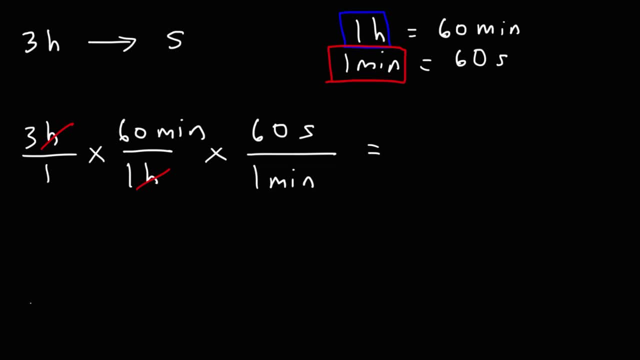 So we have one minute for every 60 seconds. So now the unit minutes cancel, So we're going to put this on the bottom. So we have one minute for every 60 seconds, And so we're left over with the unit seconds, And so we're going to multiply the numbers that. 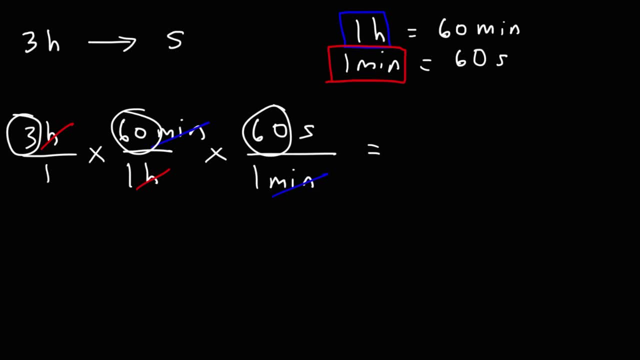 we see on top, It's going to be 3 times 60 times 60.. 60 times 60 is 3600 times 3.. That will give us 10,800 seconds. So that's how we can convert from hours into seconds. Now let's work on another. 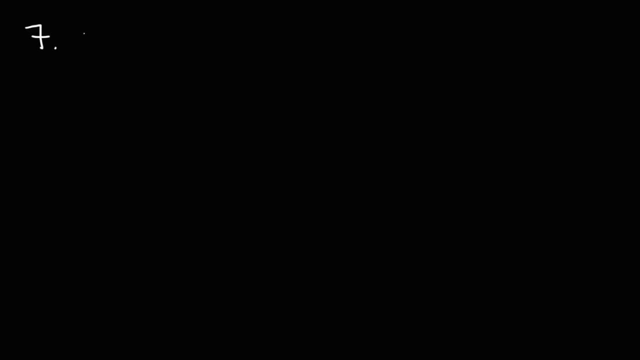 example, for the sake of practice, Let's convert 7.5 hours into seconds. So, based on the last example, go ahead and try this one for practice. So let's start with what we're given, And that is 7.5 hours, And let's write our conversion factors. 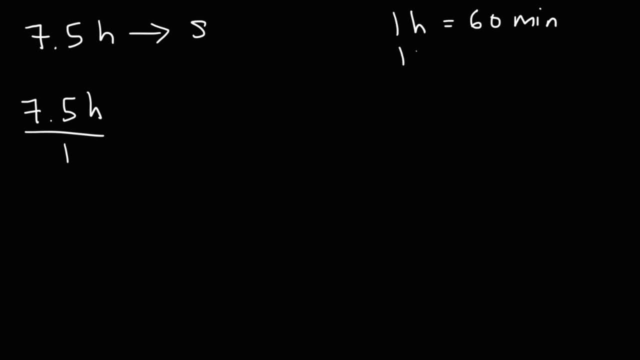 One hour is equal to 60 minutes And one minute is equal to 60 seconds. So let's convert hours into minutes first. So 1 hour corresponds to 60 minutes, And so the unit hours cancel. Now let's convert minutes into seconds. One minute is equal to 60 seconds, So now we can. 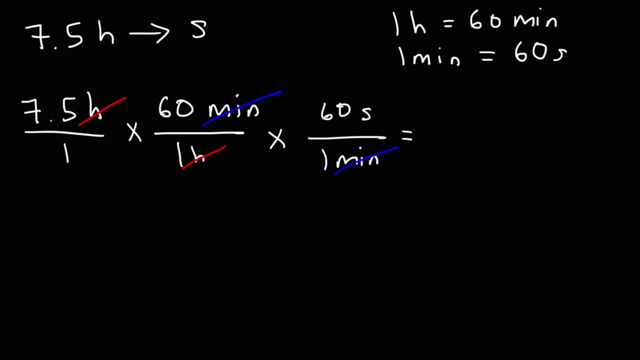 cancel the unit minutes, And so it's going to be 7.5 times 60 times 60.. Or 7.5 times 3600.. So the answer is 27,000 seconds. Now for those of you who want to get to the answer quickly, here's: 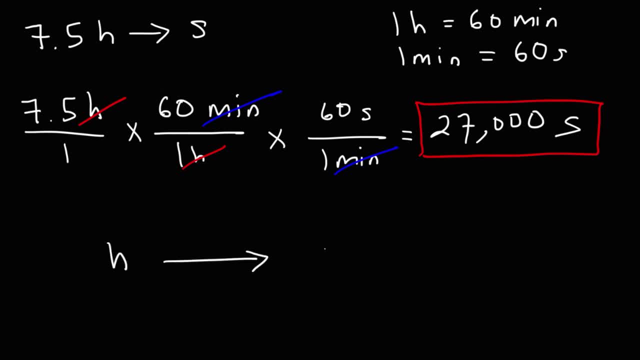 a shortcut: To go from hours to seconds, you need to multiply by 3600. And if you want to go from seconds back to hours, you need to divide by 3600.. And we're going to go through two examples of converting seconds to hours So you could. 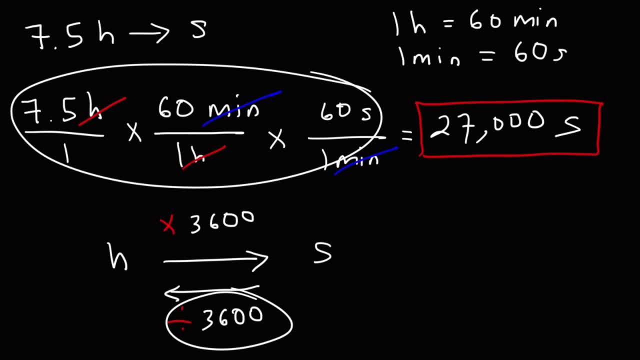 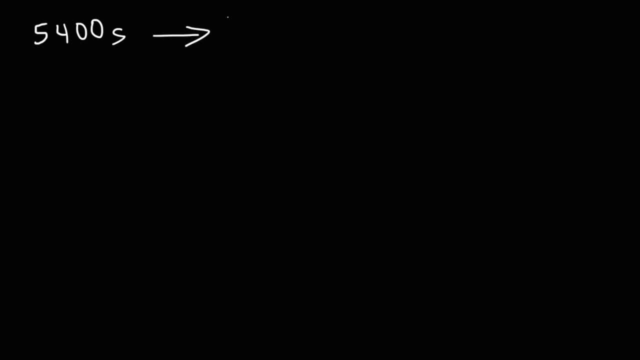 use the shortcut method, or you could show your work. it's up to you. Now, let's say that we have 5400 seconds and we want to convert that to hours. Go ahead and try that problem. So let's start with what we're given, and now we're going to. 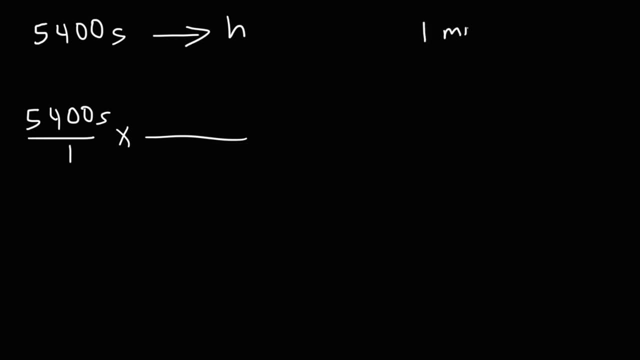 convert seconds to minutes. Keep in mind one minute is equal to 60 seconds. So what should we put on the top and what should we put on the bottom using this conversion factor? What would you say? So, since we have seconds on the top left in the first, 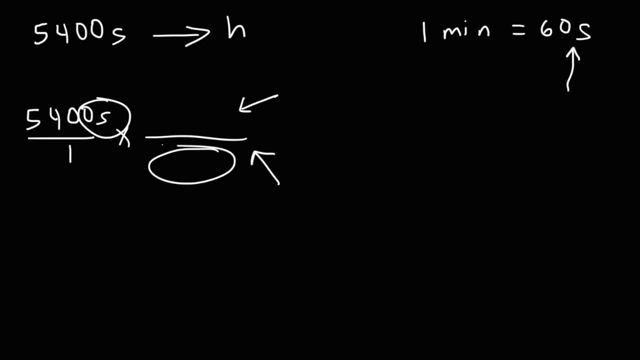 fraction. we want to put 60 seconds on the bottom right of the second fraction. So we're going to put one minute on top so that the unit seconds cancel. Now we're going to convert from minutes to hours. We know that one hour is equal to 60 minutes. 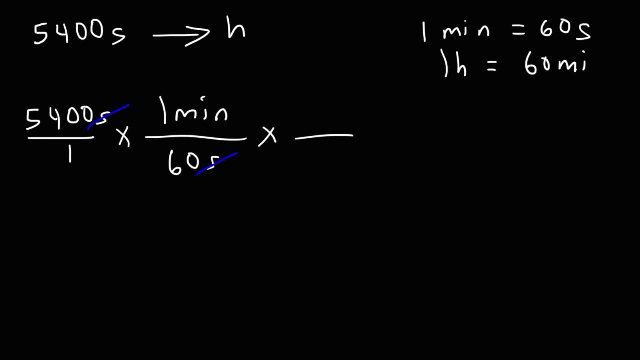 And since we have the unit minutes on top, we're going to put 60 minutes on the bottom and one hour on the top, So the unit minutes will cancel giving us the unit hours. So this time, notice that these two numbers are on the bottom: 60. 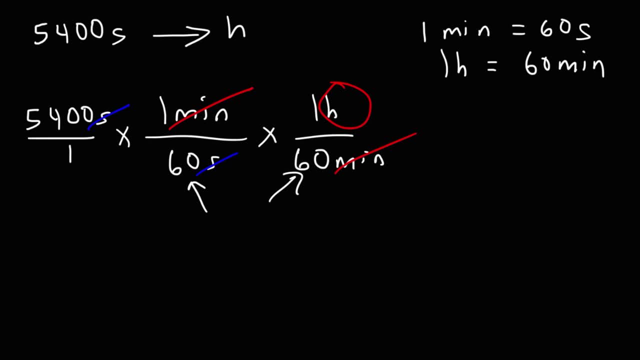 times 60 is 3600.. So it's going to be 5400 divided by 3600. Which is 1.5.. So that's the answer. 5,400 seconds is equal to 1.5 hours. Now let's try another one. 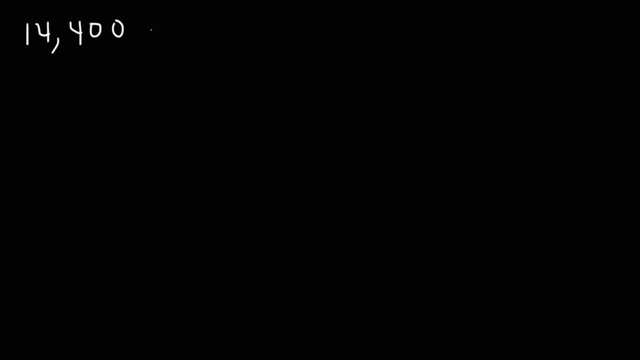 Let's say we want to convert 14,400 seconds into hours. Try that. So we're going to follow the same procedure. First we're going to convert seconds into minutes- One minute is equal to 60 seconds- And then we're going to convert minutes into hours. 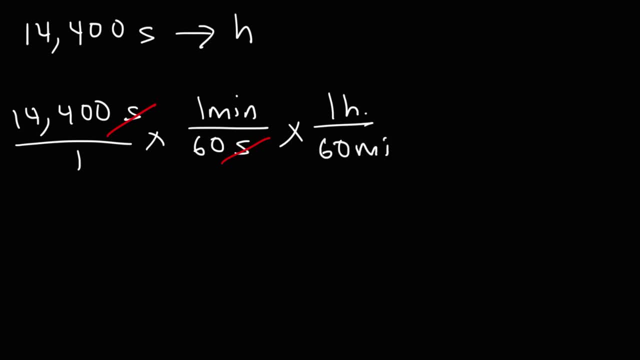 One hour is equal to 60 minutes. So now we could cancel the unit minutes, And so it's going to be 14,400 divided by 60, which is 240.. And then take that divided by 60 again, So that will give you four hours. 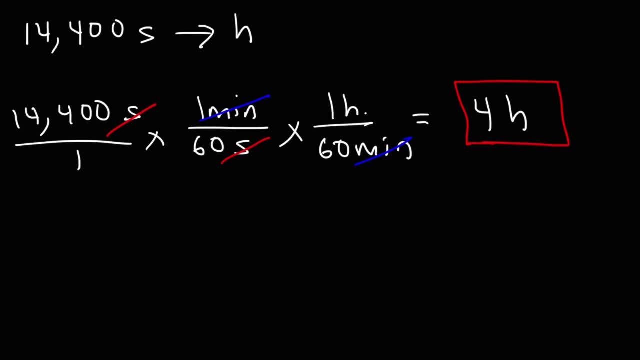 So, as you can see, it's not too difficult to convert from seconds to hours And hours to seconds. But here's a question for you. Let's say, if you were given six hours and 40 minutes, How would you convert that into seconds? 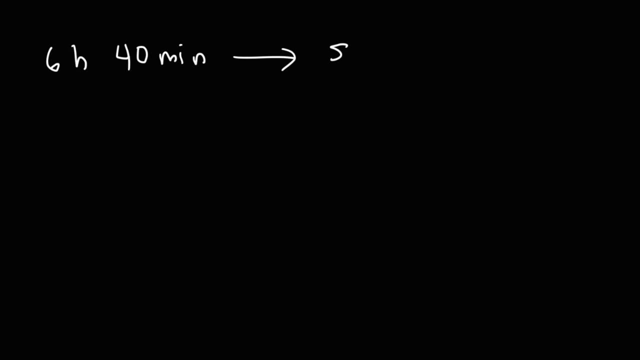 Feel free to pause the video and try that example Now. it's helpful to know that one hour is 3,600 seconds, Because you got to do 60 times 60 to get from hours to seconds And we know that one minute is 60 seconds. 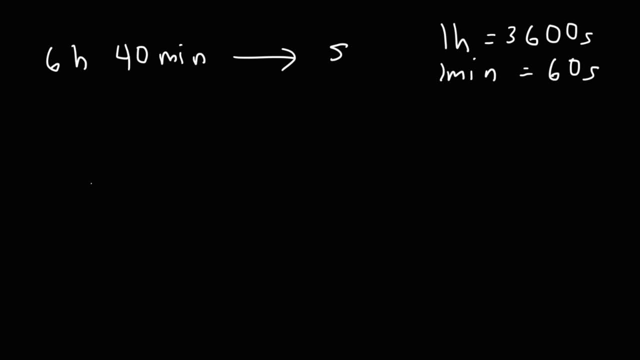 So what we're going to do is we're going to convert each part separately into seconds. So let's start with six hours. So we have 3,600 seconds for one hour. So for six hours it's just going to be six times 3,600.. 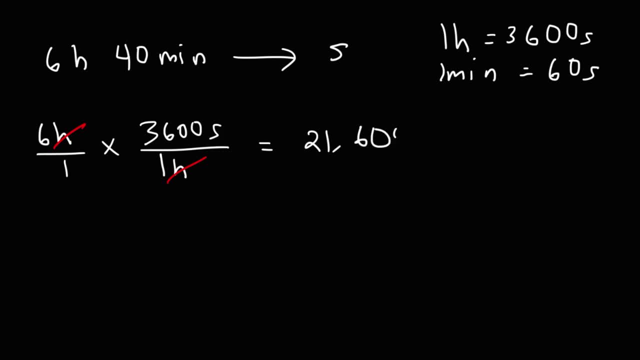 And so that's going to give us 21,600 seconds. Next, let's convert 40 minutes into seconds, So there's 60 seconds in each minute. So in 40 minutes it's going to be 40 times 60.. 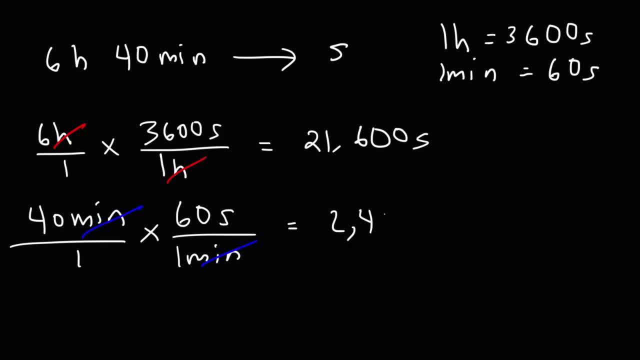 Which is 2,400 seconds. So now all we need to do is take the sum of those two values, So let's put a plus sign. So 21,600 plus 2,400 gives us a total of 24,000 seconds. 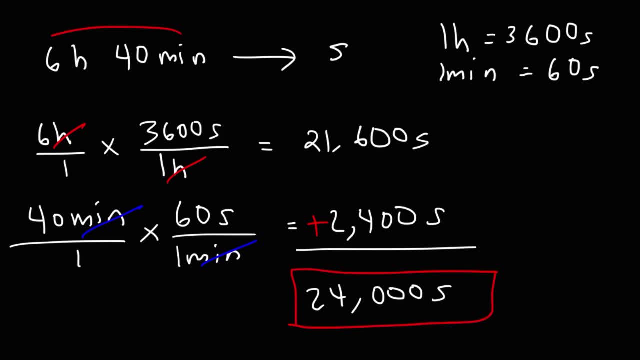 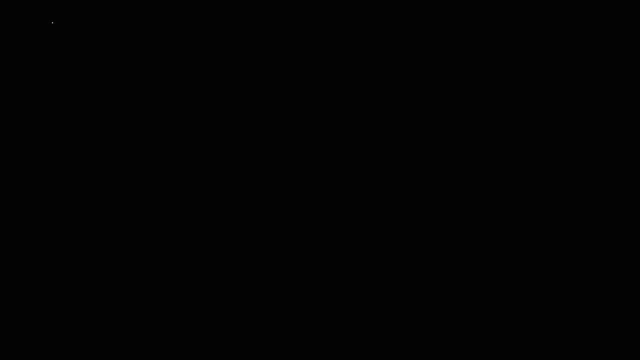 So this is equal to six hours and 40 minutes. Now, for the sake of practice, let's try another example. Let's say we have eight hours and 25 minutes. Go ahead and convert that into seconds. So let's follow the same process. 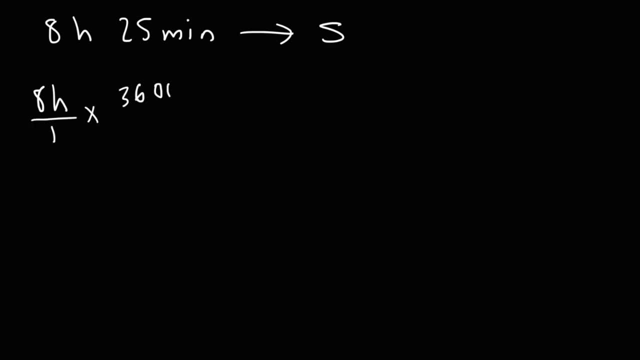 Let's begin by converting hours into seconds. So we have eight hours and 26 seconds. Keep in mind, one hour contains 3,600 seconds, So this is going to be eight times 3,600. And that is 28,800 seconds. 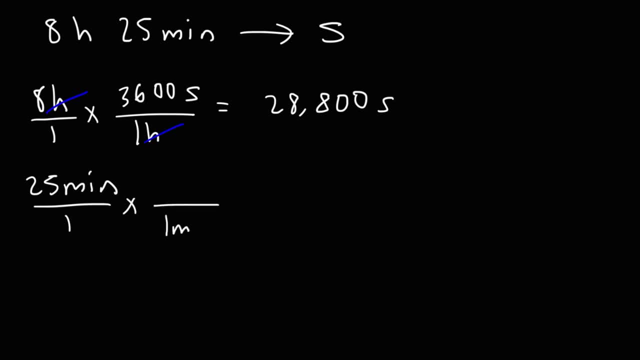 Next, let's convert 25 minutes into seconds, And each minute contains 60 seconds, So it's going to be 25 times 60 seconds, And so you should get 1,500 seconds. Now let's add those two numbers. 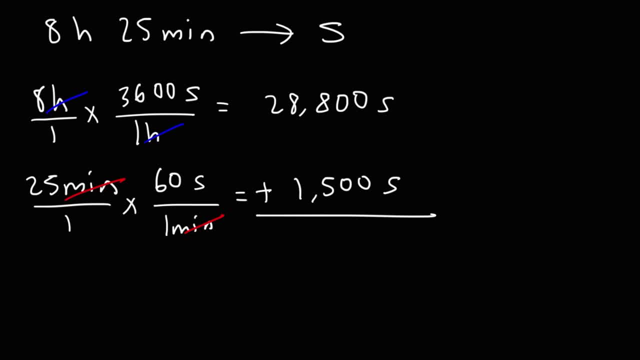 So 28,800 plus 1,500. This will give us a final answer of 30,300 seconds. So that's how you can convert from hours and minutes into seconds. Now what if you are given 30,300 seconds? 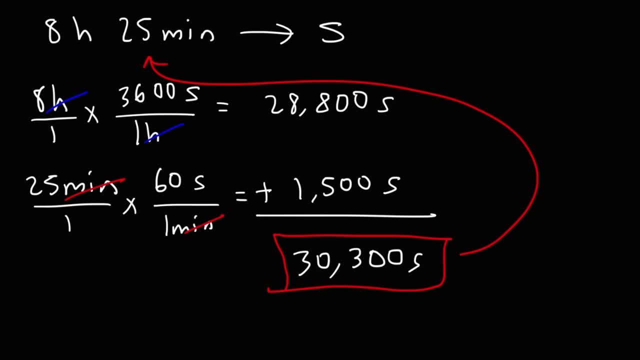 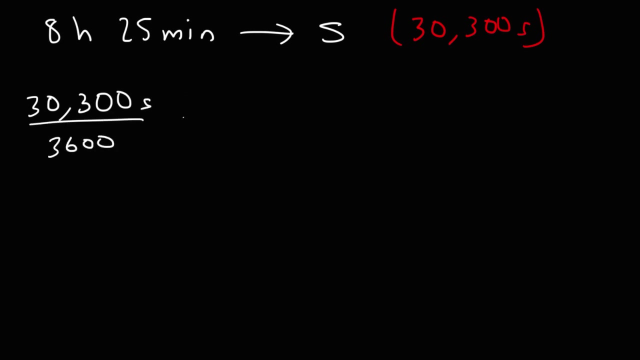 Can you use that To go back to this answer? eight hours and 25 minutes. Let's see if we can do that. So I'm going to put this here. So the first thing you want to do is you want to take this number and divide by 3,600. 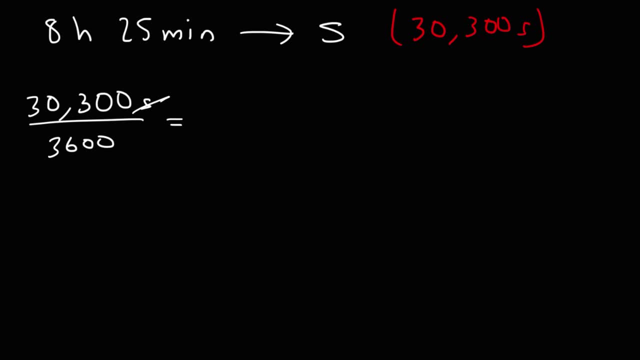 Let's not worry about the units for now. So this will give you 8.416 repeating. So we're going to take the number in front of the decimal 8, and that's going to go in front of the unit hours. 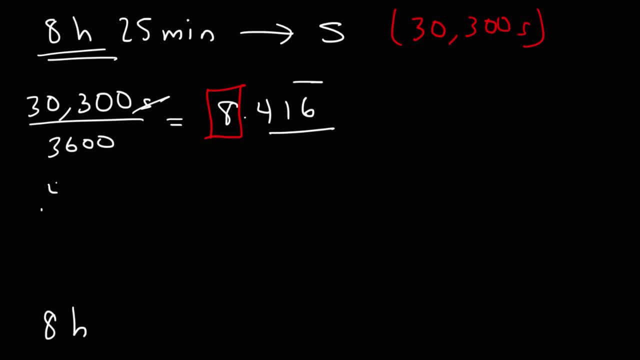 So that's our 8 hours, right there. Now what remains? The 0.416, repeating which you can write that as 0.4166667.. Multiply that by 60. And you should get 25.. So that will give us the 25 minutes part.